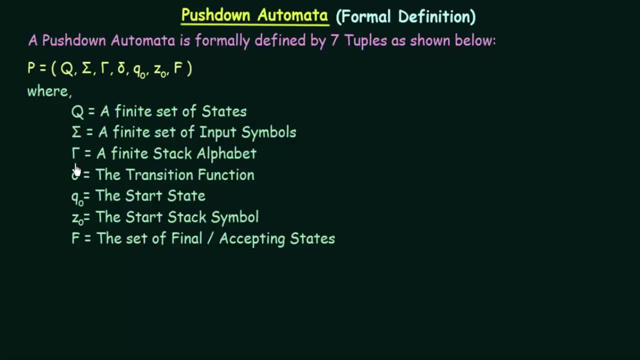 And then we have uppercase Gamma, or capital letter Gamma, which represents a finite stack alpha. So this is something which was not there in our finite automata And I told you even in the previous lecture: what makes the push-down automata different from the finite automata is the presence of a stack. 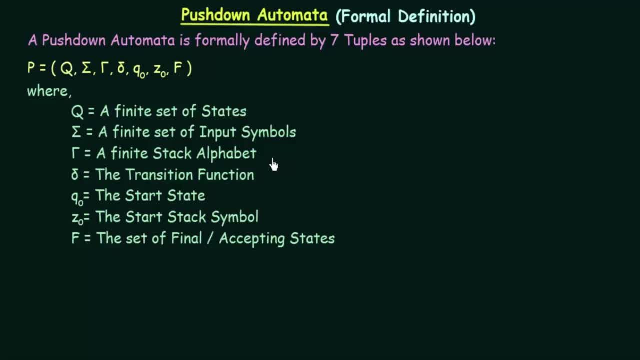 And the stack is what makes push-down automata more powerful than the finite automata. And then this capital letter Gamma, or uppercase Gamma, is a tuple that is used to denote the finite stack alphabets or the symbols That are present in the stack. 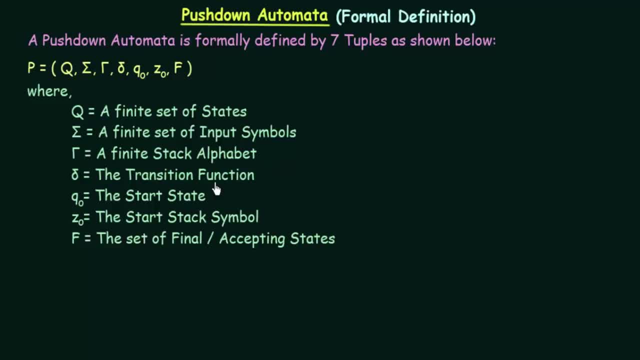 And then we have Del, which represents a transition function, And, if you remember, in the finite automata also we had Del, which represents a transition function, and the transition function had a specific meaning. And even in this push-down automata also this transition function will have a specific meaning, which I will be explaining as we go further. 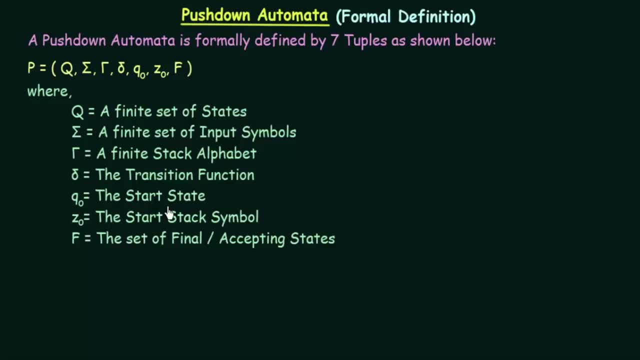 And Q0 is the start state. This is also same like our finite automata, Where Q0 represents the start state or the initial state, And then Z0 it represents the start stack symbol. So this is also something that was not there in case of finite automata. 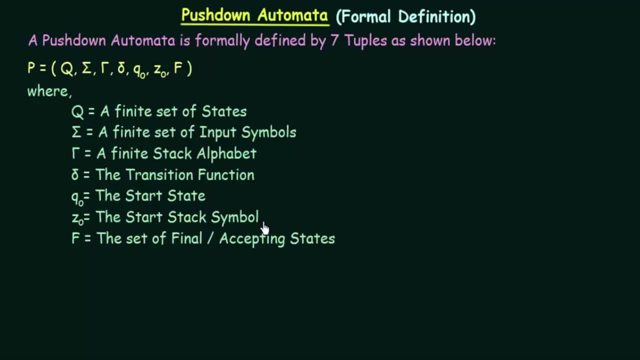 So, in case of push-down automata, as I already taught you, we are having a stack in this And then Z0: it represents the first symbol, or the start symbol that is present in the stack, And then, finally, we have F, which is the set of final state or accepting states. 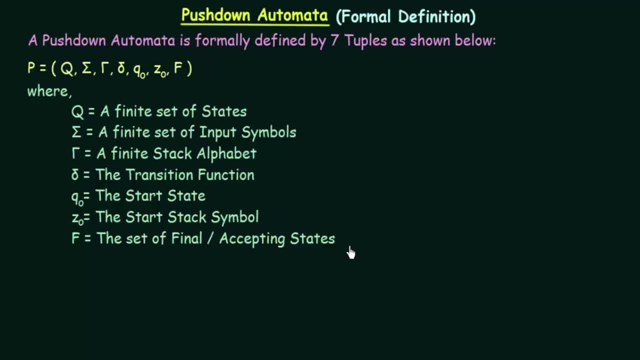 So this is also same, like our finite automata, where the letter F is used to denote the set of final states or accepting states. So I hope those tuples were clear to you. Now we need to talk about the transition function, which is denoted by Del. 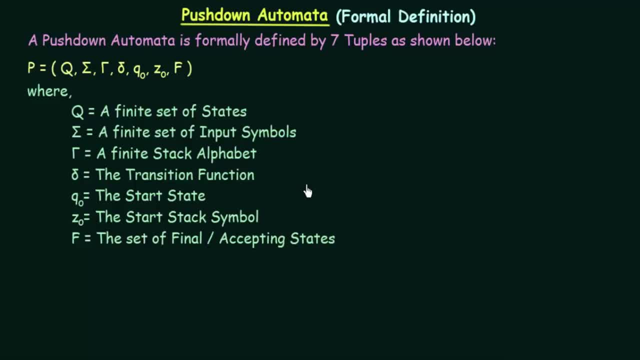 So let us see what this transition function means and how is it actually defined. So the transition function which is denoted by Del, The transition function which is denoted by Del. It takes as arguments a triple which are Q, A and X. 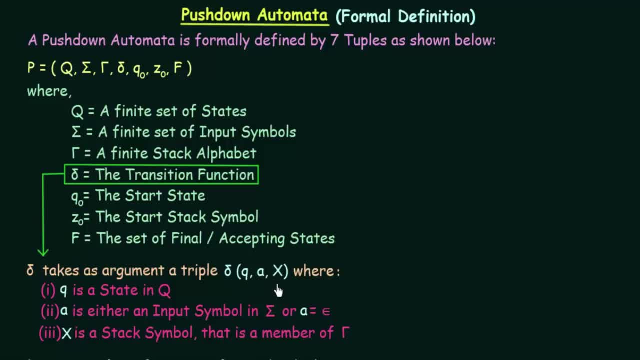 So it takes three arguments, namely Q, A and X. And let us see what this means. First one is Q. Q is a state in capital Q. So I already told you that Q, this capital Q, it represents the set of states. 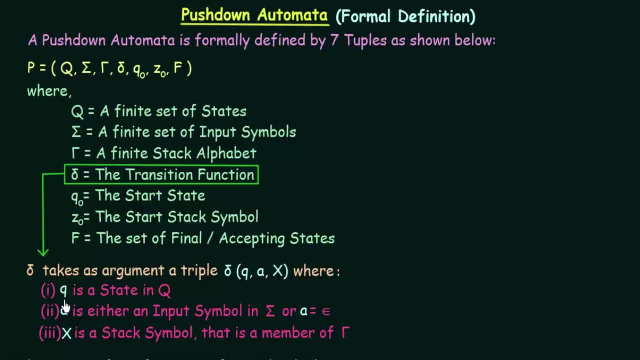 And this small letter Q. It just denotes one of the states from the set of states that we have in Q. And then A. A is either an input symbol in sigma or A is equal to epsilon. So that means that this A it could be an input symbol from our set of input symbols that we have. 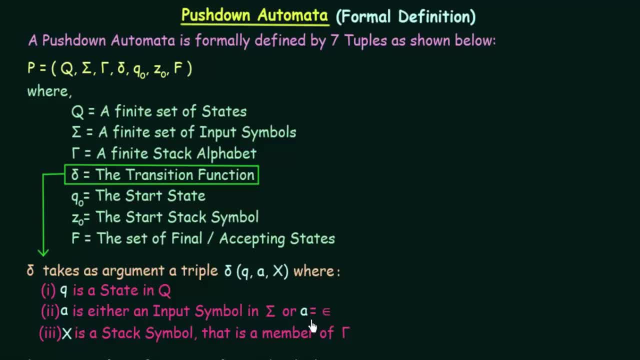 Or it can also be epsilon. That means it can also be an empty symbol. So this A can either be an input symbol Or it can be just an empty symbol. Then we have X. X is a stack symbol that is a member of gamma. 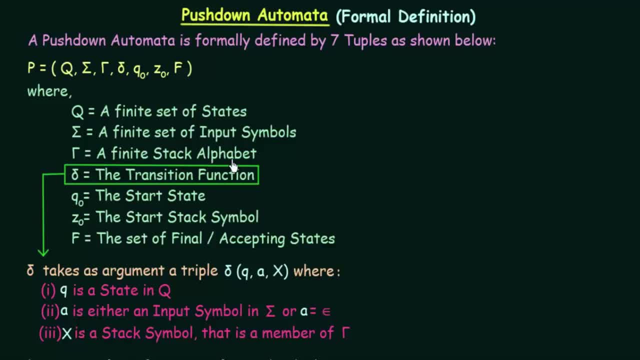 So I told you, gamma is the finite stack alphabet, The set of alphabets that we have in the stack, And X is symbol that is present in the stack. Now let us see an example of this so that it will become more clear to us. 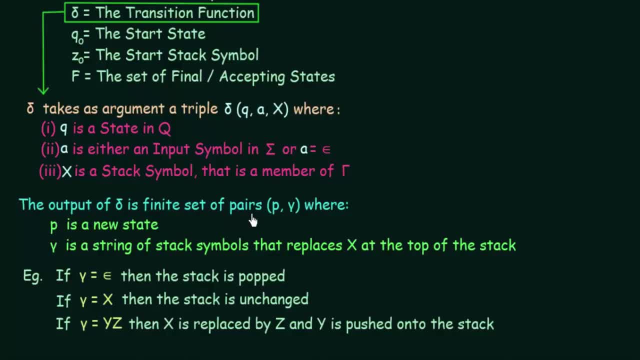 Now the output of Del. It is a finite set of pair given by P And small letter or lower case gamma. This symbol is a lower case gamma. So the output of transition function Del. It is given by a set of pairs given by P and gamma. 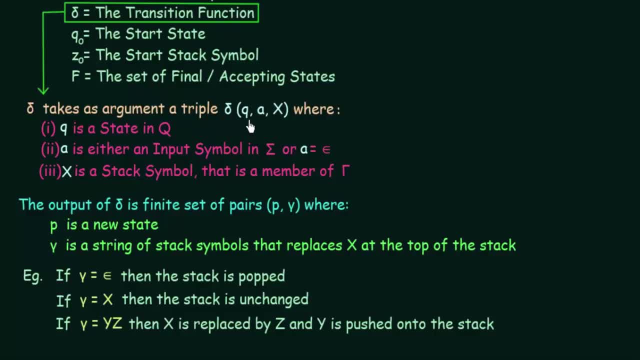 So I told you that, the transition function, it takes these three arguments, Q, A and X, And it gives an output of the form P, gamma. And let us see what this P and gamma means. P is a new state, So P is a new state from a set of states. 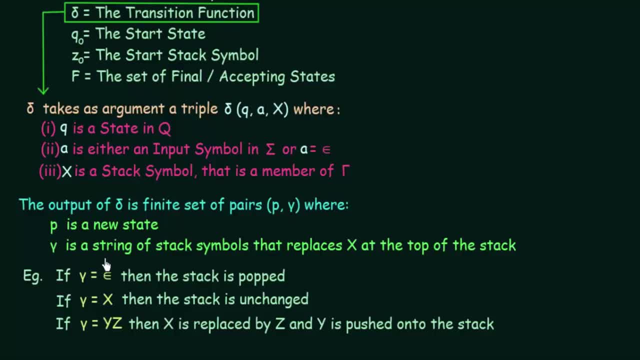 And let us see what is gamma. Gamma is a string of stack symbols that replaces X at the top of the stack. So in our input, or in our argument, initially we had X, which was a symbol from our stack, And then this gamma, which comes as an output of the transition function. 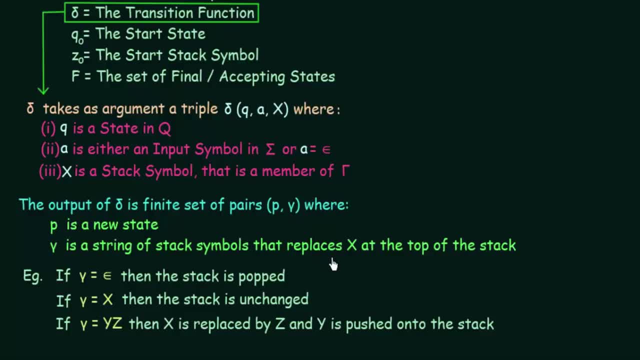 It is a symbol that replaces this X from the top of the stack. Now let us see an example to make it more clear. So if we have gamma equal to epsilon, Then it means that the stack is popped. Now, what do we mean by this? 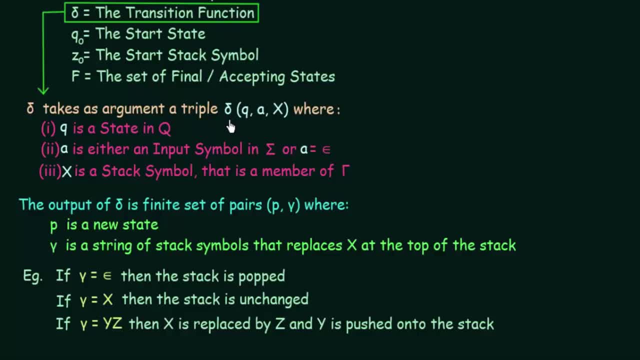 So let us say that initially, this transition function Del, It took these three arguments, Q, A and X, And it gave the output P and gamma, And P is any state. And then, in case of gamma, If gamma happens to be epsilon, 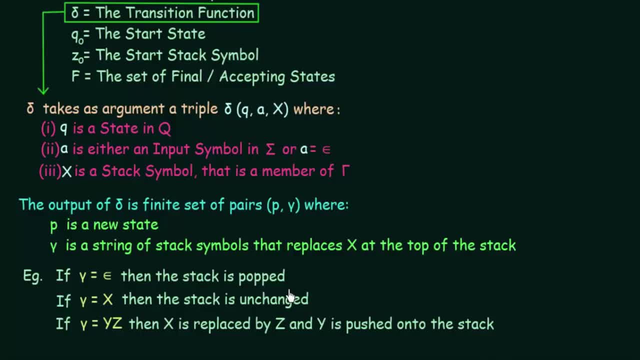 That means the stack is popped. So what do I mean by popped? I already taught you in the previous lecture that popping an element from a stack means removing an element from the stack. So if we have a stack and if all the elements are removed, then what do we have in the stack? 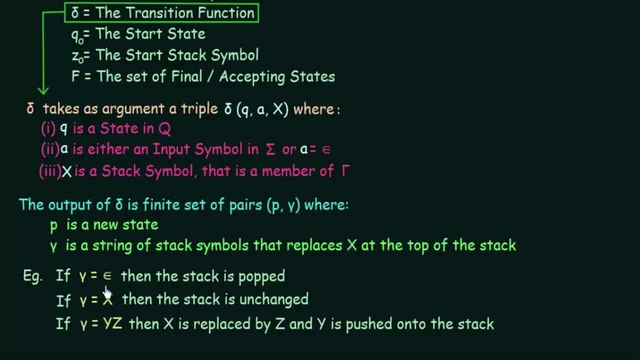 We have nothing left in the stack, So epsilon means it is empty. So if gamma equal to epsilon, that means the stack is popped, That means the elements in the stack was removed and it is empty. And now what if our gamma is equal to X? 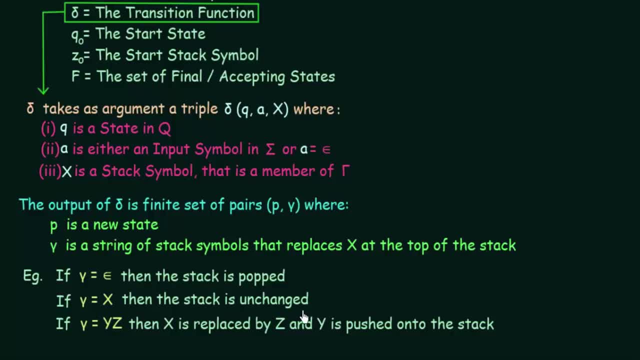 Then it means that the stack is unchanged. Now, why is this? This is because initially, we knew that the symbol or the element in the stack was X, And then the output that we get is gamma, And if gamma is equal to X, that means the element in the stack is unchanged. 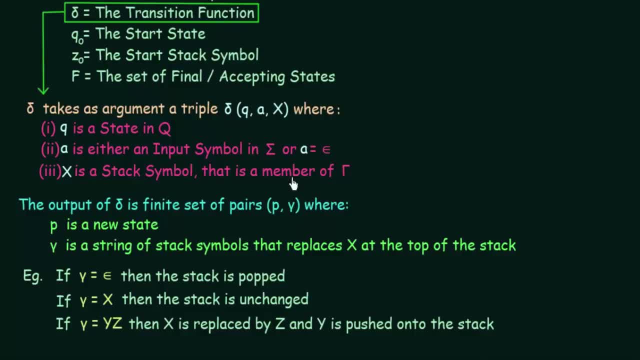 We did not make any change in the stack Because initially it was X and finally also gamma is equal to X. So if gamma is equal to X, That means the stack is unchanged. And finally, if we have gamma equal to YZ. 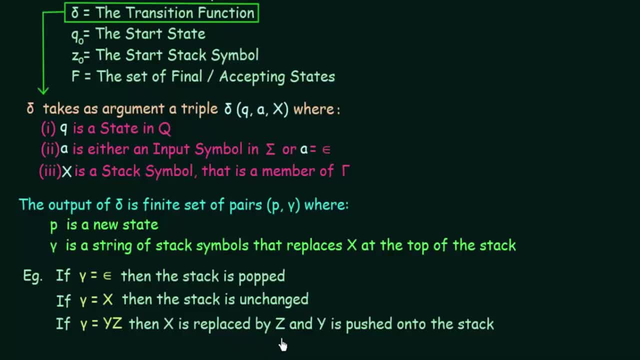 Then it means that X is replaced by Z and Y is pushed onto the stack. So if we take this as the initial argument, If this was the argument that we have in our transition function, And as an output, if we get gamma equal to YZ,